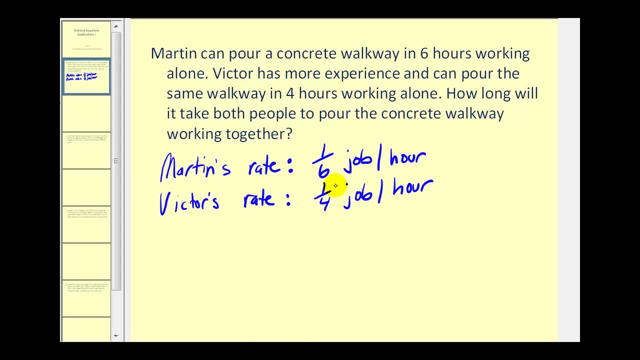 Since they'll be working together, we're going to be adding their rates together. So if we let t equal hours, then in any t the fraction of the job that would be complete would be Martin's rate times the number of hours plus Victor's rate times the number of hours. 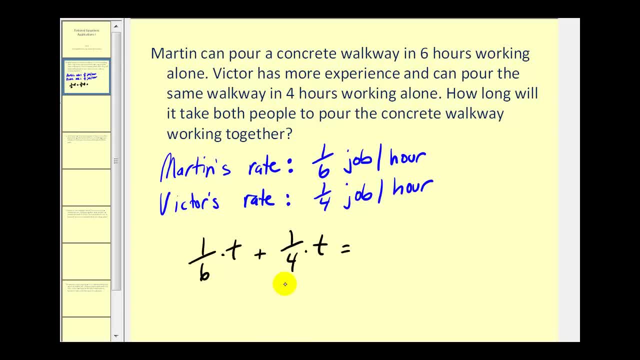 Since we want to know when this job would be one hundred percent complete. one hundred percent as a fraction would be equal to one, And this is the equation we need to solve in order to determine how long it will take if they both work together. 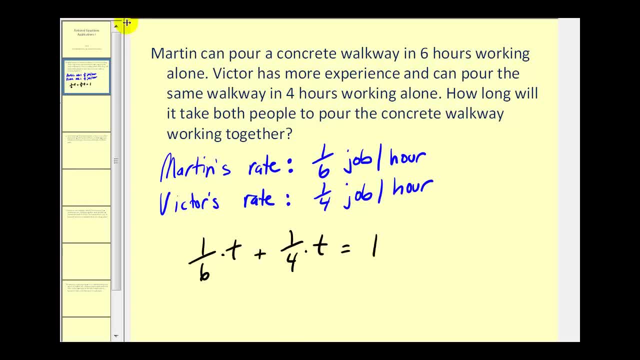 Let's go ahead and take this over to the next Now. if we wanted to, we could rewrite this as t over one and t over one. So we could write this equation As: t over six plus t over four must equal one. Let's go ahead and take this equation over to the next screen and then solve for t. 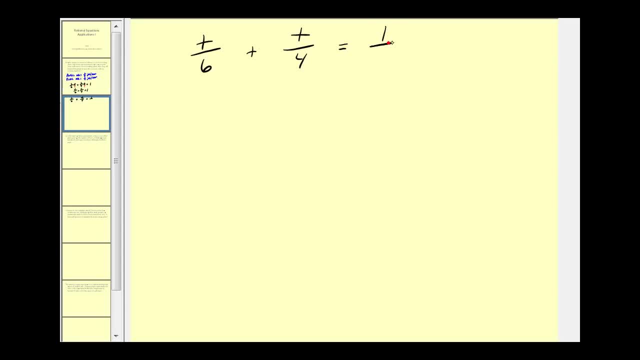 I'm going to go ahead and rewrite one as one over one, And what we'll do here is we'll clear the fractions by multiplying every term by the LCD. Well, the LCD would be twenty-four, so we'll multiply each term by twenty-four over one. 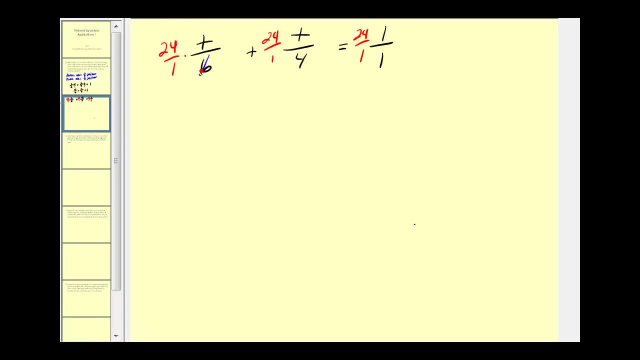 Now, before we multiply, we'll simplify. This would change to a one. This would be four. So I'll have four t. Here we have a common factor of four. That would change to a one. That would be a six Plus six. t must equal twenty-four. 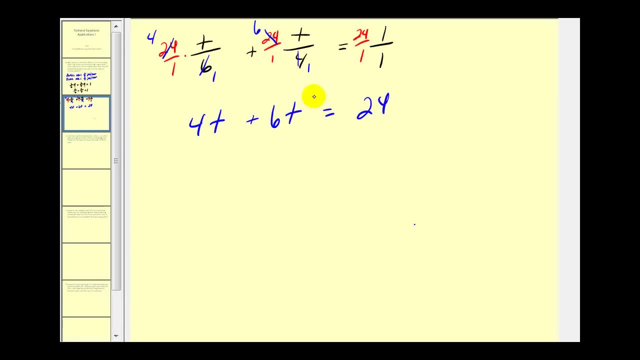 So now we'll solve this equation. for t, This would be ten. t equals twenty-four. Dividing both sides by ten, T equals this would be two point four hours. If they work together, they can complete the job in two point four hours. 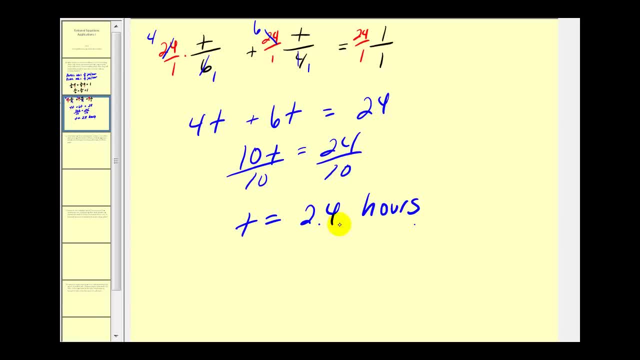 Now if we want to know specifically how many minutes we could convert point four hours into minutes, Let's go ahead and do that Point four hours over one. Multiply this by sixty minutes over one hour. Notice how the units of hours simplify out. 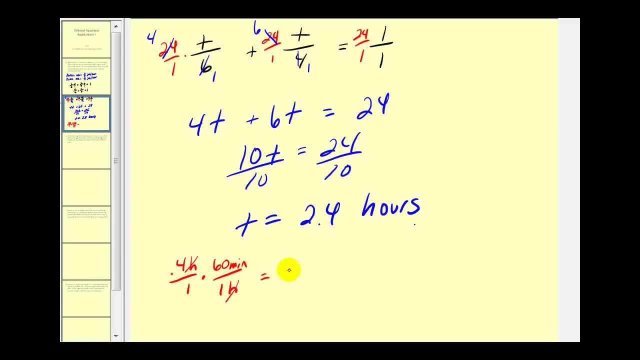 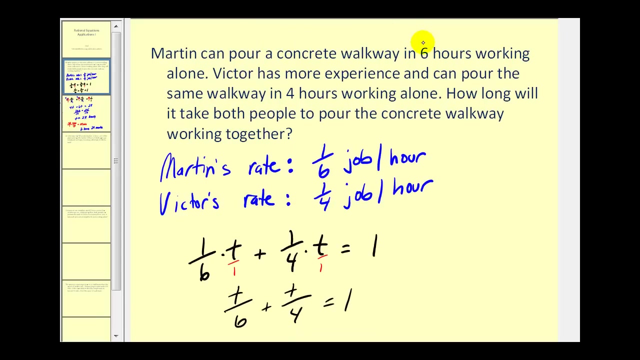 Point four times sixty would be twenty-four minutes. So more specifically, the total time to complete the job, if they work together, would be two hours twenty-four minutes. Now that should make sense because if we go back to the original problem, if Martin can complete the job in six hours and Victor can complete it in four hours. 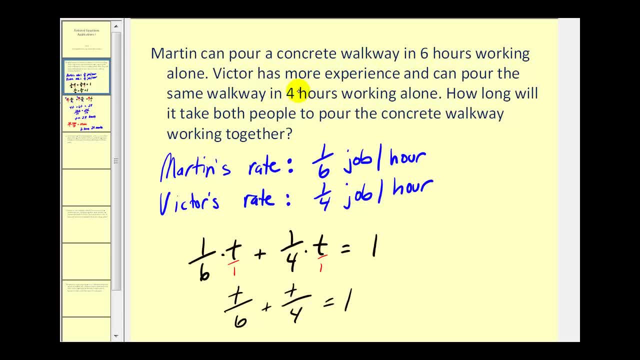 of course, if they work together it should be faster than the fastest person, So having an answer less than four hours does make sense. Let's go ahead and take a look at another problem. An inlet pipe can fill a tank in twelve hours. 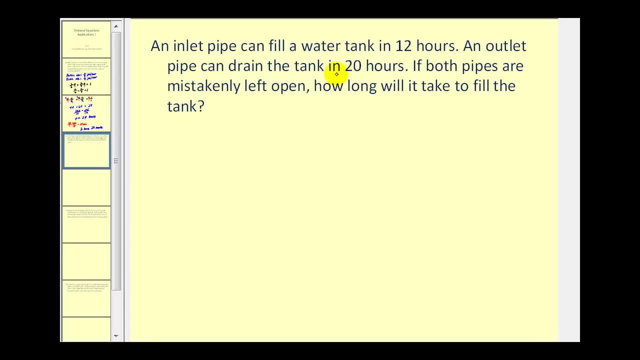 An outlet pipe can drain the tank in twenty hours. If both pipes are mistakenly left open, how long will it take to fill the tank? So what's happening here? we have water coming in and also water going out. Let's go ahead and determine the rates. 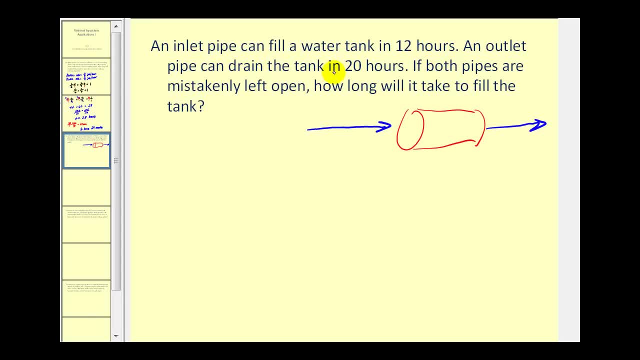 If it takes twelve hours to fill the tank, the rate of the water going into the tank would be one-twelfth of the tank per hour. And if it takes twenty hours to drain the tank, the rate of the water leaving the tank would be one-twentieth of the tank per hour. 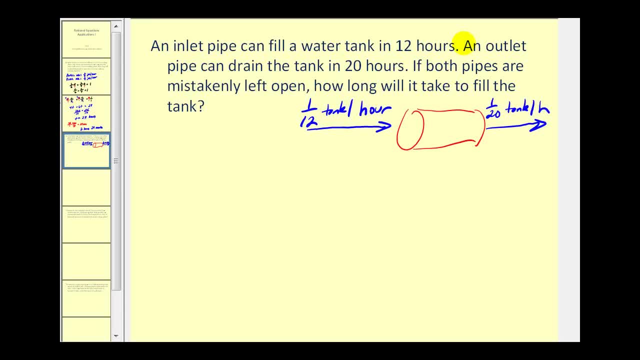 So again, if you let t equal time in hours, we can write an equation to represent how much water would be in the tank at any time. In this case they're working against each other. So this is the rate of the water going in. this is the rate of the water going out. 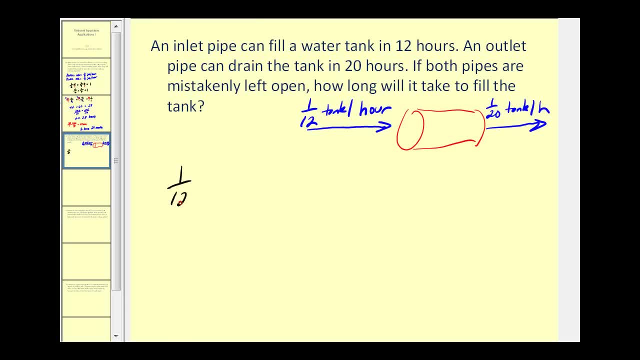 So the equation that we would come up with would be one-twelfth times the number of hours, and it would be minus one-twentieth times t. Now again, at any time. t. this would represent what fraction of the tank would be full. 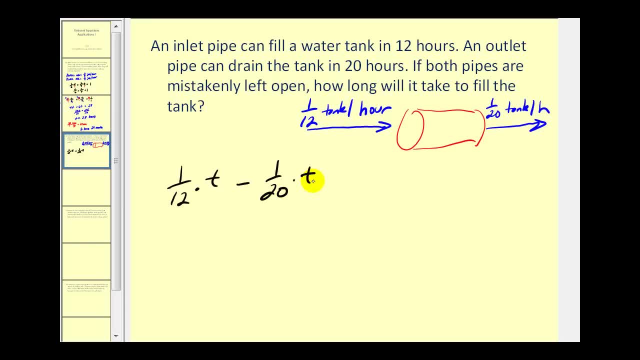 But since we want to know when the tank would be full or one hundred percent full, as a fraction that would be equal to one or one over one, Let's go ahead and rewrite this one more time and then we can solve it. 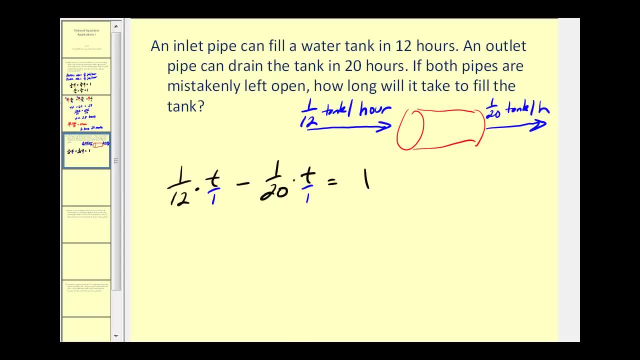 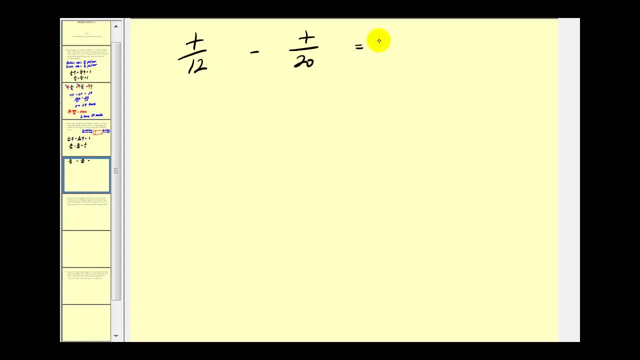 Again, these t's could be written over one. So the equation that we can set up and solve now would be: t over twelve minus t over twenty must equal one over one Again. let's take this to the next slide, where we have more room.